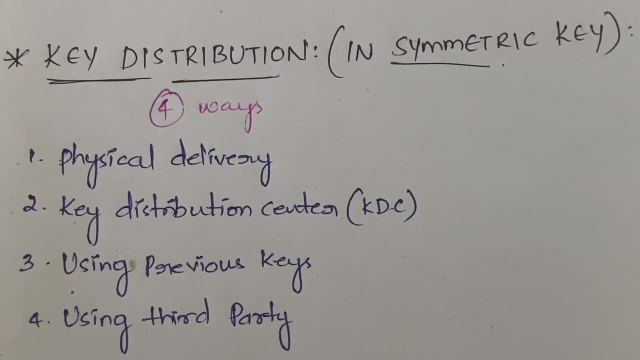 So here, how you do the key distribution in case of symmetric key. we are going to learn the subject of network security, Got it? So we have total of four ways to do this. The first one is the physical delivery. This video is going to be very short, a theoretical video, very simple, very short and easier video. 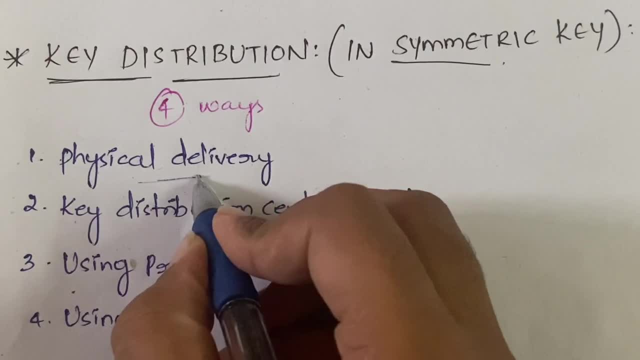 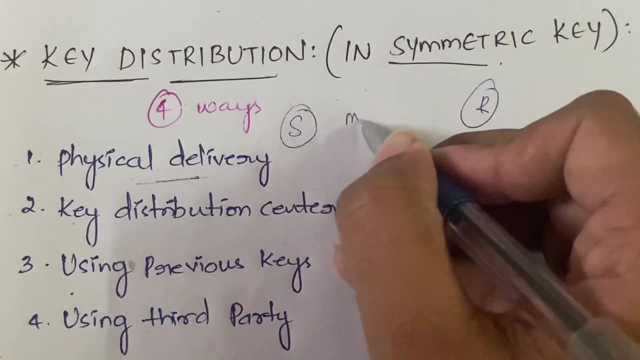 Okay. so first is: it is the physical delivery. physical delivery in the sense, what you will do is suppose you are the sender and you have the receiver. Okay, the sender and receiver will meet physically, that is, you will be going to the sender's place, or receiver will be coming to your place, or you'll be meeting at a cafe or somewhere. 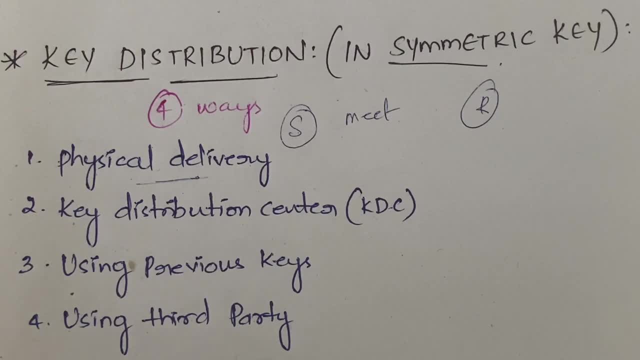 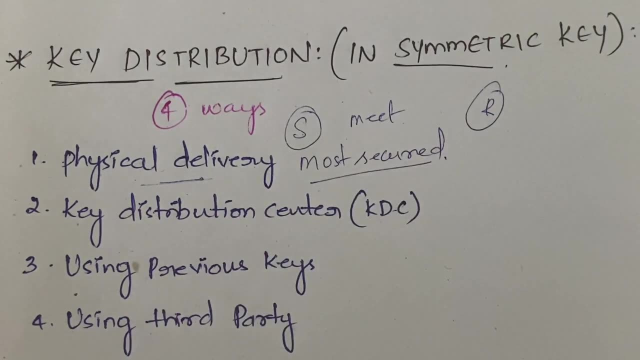 You will be meeting physically and exchanging the key. So therefore it is the most secured algorithm- Algorithm in the sense, not algorithm- actually- more secured way in which you can share the key. Got it Because you you are directly going, you're directly meeting the receiver or the receiver is directly meeting the sender. 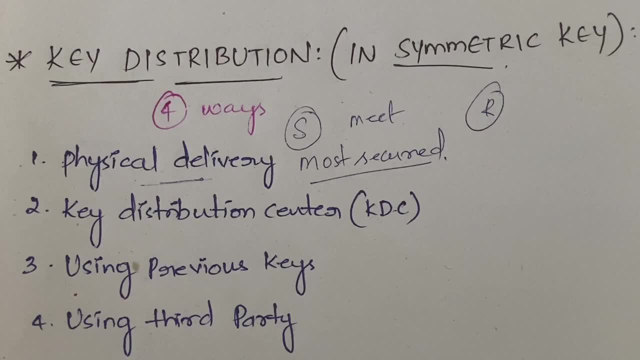 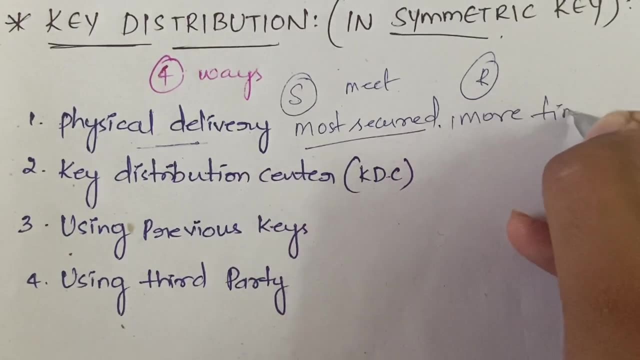 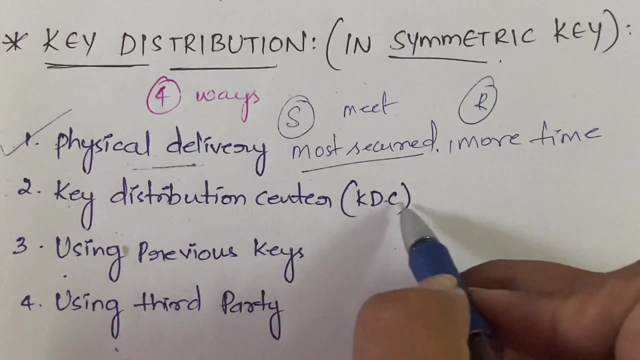 There is no chance for the loss of the key to the third person, Right? So? but in spite of being more secured, it has a disadvantage, that is, it takes more time. That is obvious, Right. Traveling time, waiting time, all will count, Got it. So this is the physical delivery, And the second step is we have the KDCs. 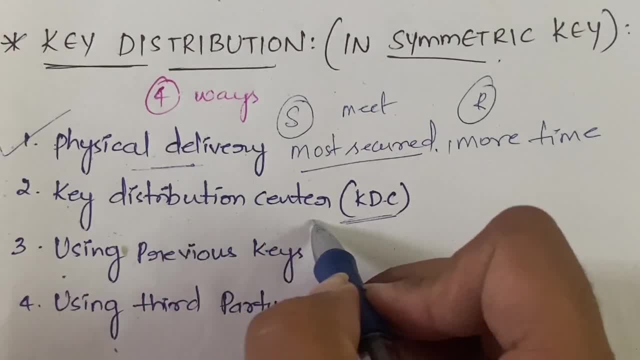 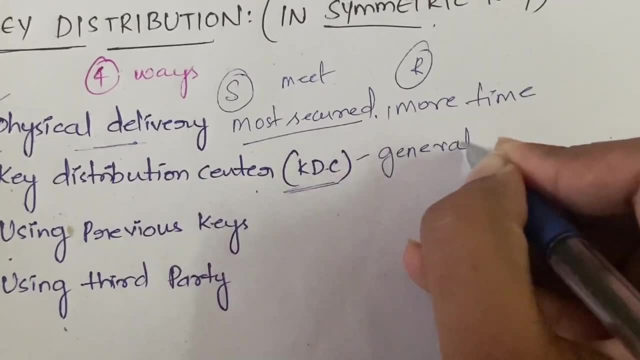 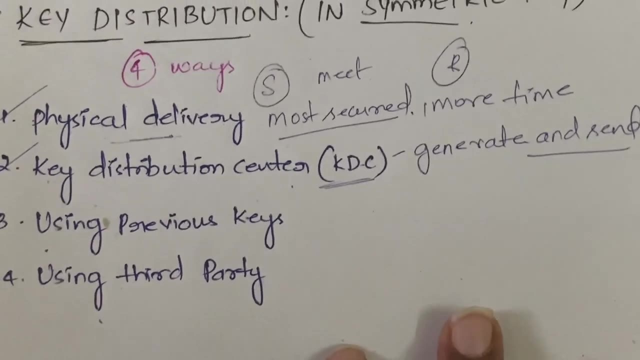 KDC is nothing but the key distribution center- Got it. So here what happens? is this KDC? what it does is it will generate the key. It will generate the key and it will send the key to the sender and the receiver, both. It will send the key to the both sender and receiver Got it. 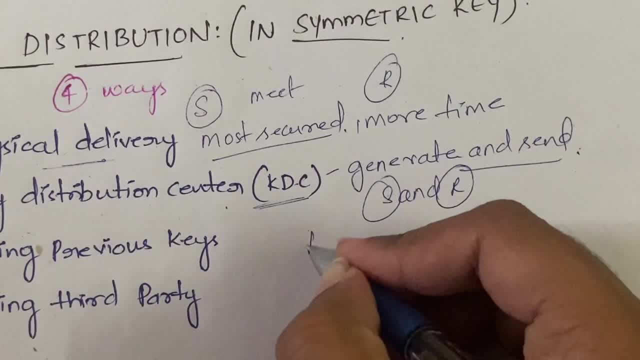 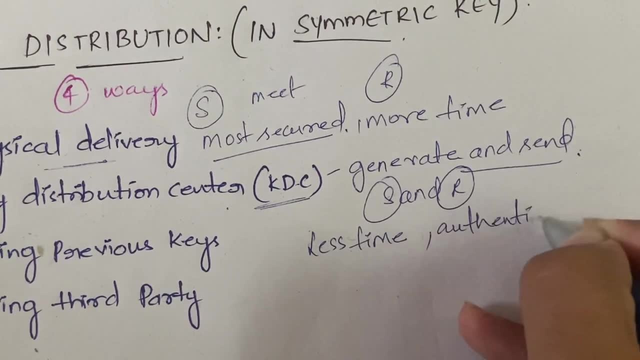 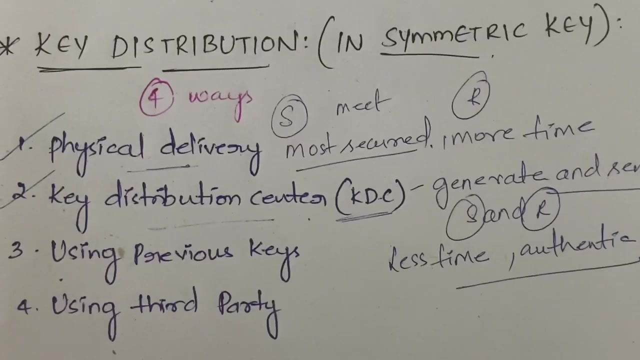 And here it is. it takes less time because no physical work is involved here, and it is authentic, Got it. But here you have to rely on the third party. You have to rely on some KDCs, some key distribution center. You have to depend on them, Got it. 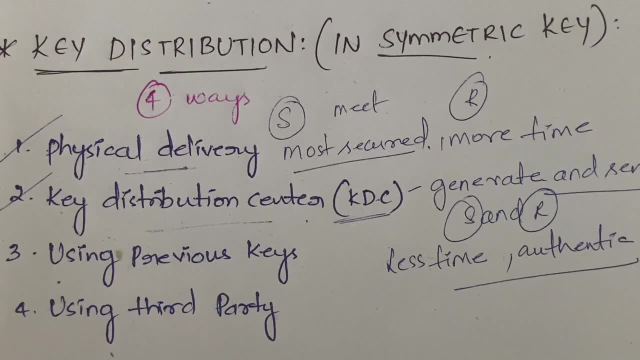 So it is taking less time, It is authentic and you need to depend on the third person. And in case of key distribution centers, the key distribution center itself will generate the key. it will distribute it to both sender and the receiver as well got it, and the third step is.